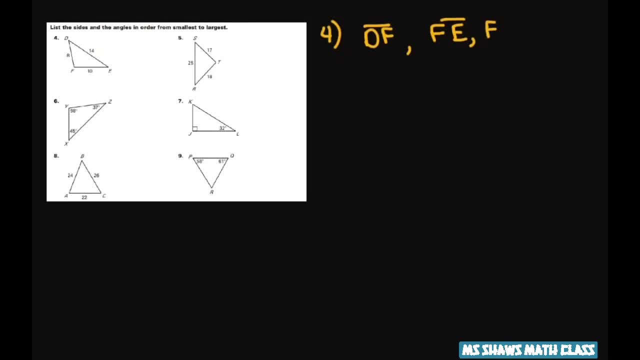 And the next one is ED. So that's just based off these numbers here. So for the angles, we go from the smallest side to the angle across from that side. So this would be angle E, FE. this side goes across here and that would be angle DF. 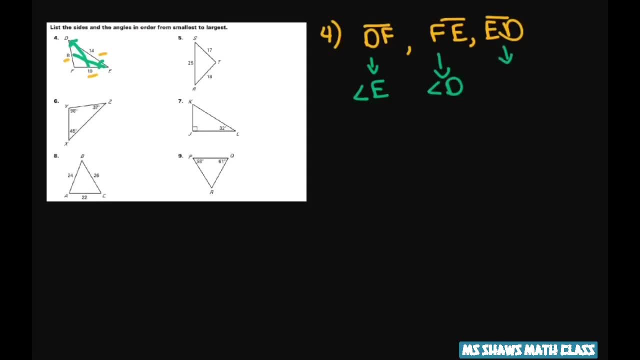 And then ED, that goes to angle F. All right, and then do the same thing with the next one. The smallest side for five would be ST, Then you have TR, Then you have RS And then you just go to the side opposite. 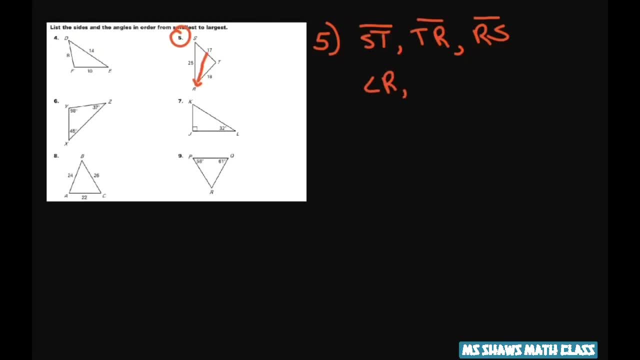 and write the angle. So that's AD, So that's angle R, Then 18 goes to angle S And 25 would go to angle T And the next one. we have the angles. So let's do the angles first. For number six, angle Z. 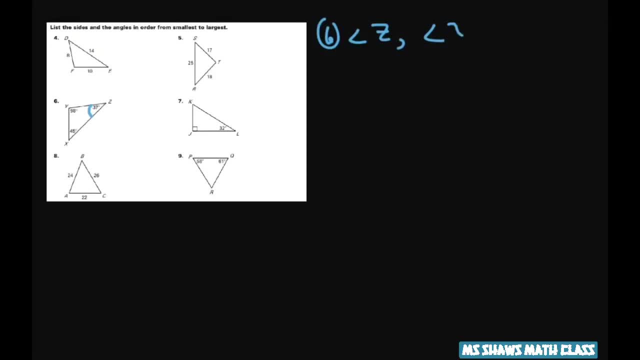 is the smallest, And the next is angle X, The next is angle Y, So now we go to the sides, across from it to get the smallest. So across from Z is XY, Across from X is YZ And across from Y is XZ. 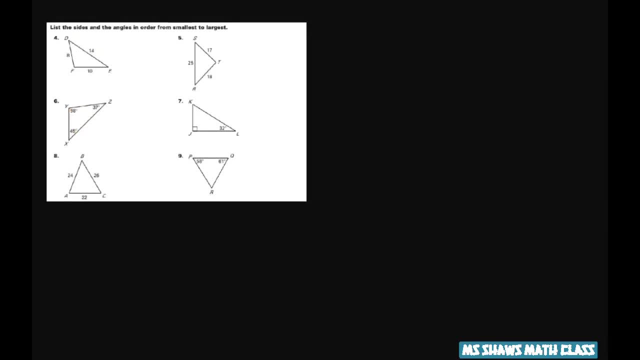 All right, And for this one it's X one. I need to figure out what that is. just take 90 minus 32, which gives you 58. so I just took 90 degrees minus 32 and this angle would be 58 here. so the 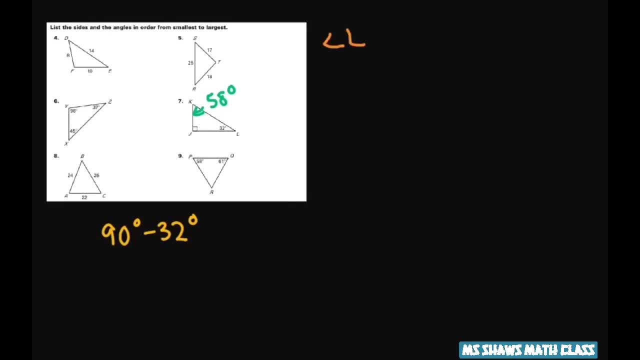 smallest is 32, which is angle L, the next one is angle K, which is 58, and then angle J is 90 degrees. now let's go across from L. that side is going to be KJ, cross from K is JL, and across from the 90 degrees is KL. 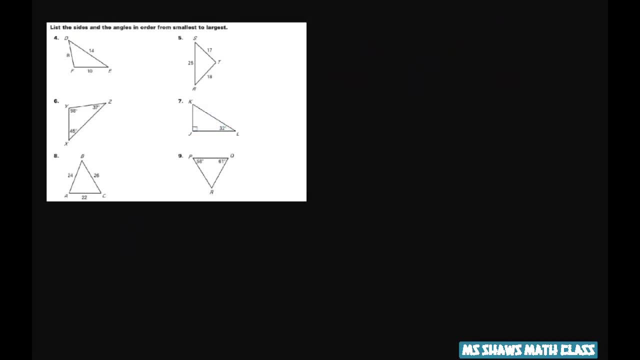 okay, and you might want to try the next ones on your own. we just do the smallest, that's AC and then AB and then BC. now just go across from 22 degrees, that would be angle B. cross from a, B is angle C, and across from BC is angle a. and now we have to get this one, since 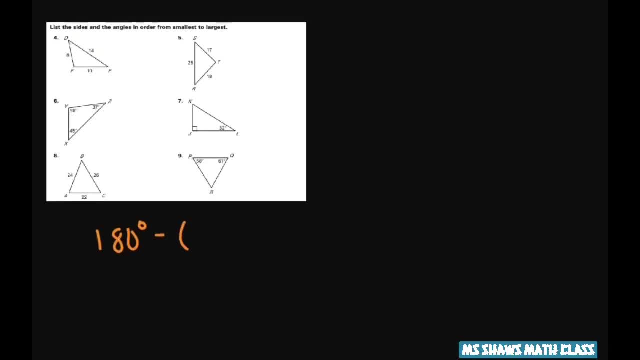 it's going to be 180 degrees minus 58 degrees plus 61 degrees, so 58 plus 61 is 119. so subtract that from 180, you get 61 degrees. so this one is 61. so let me just double-check that. alright, so we have two that are the same. so our smallest angle. 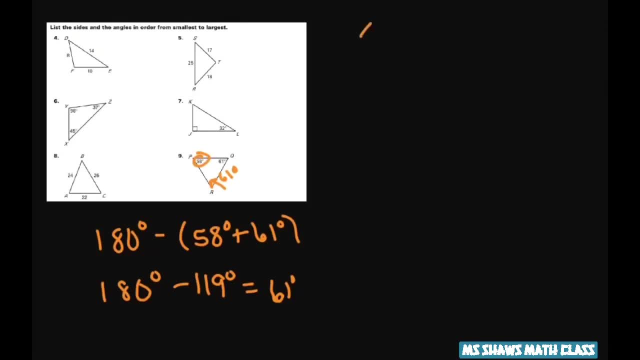 is is 58.. It's angle P And the other two. this is apparently they're the same. So just say angle Q and angle R are the same length. So for P, the side across from that is going to be RQ.